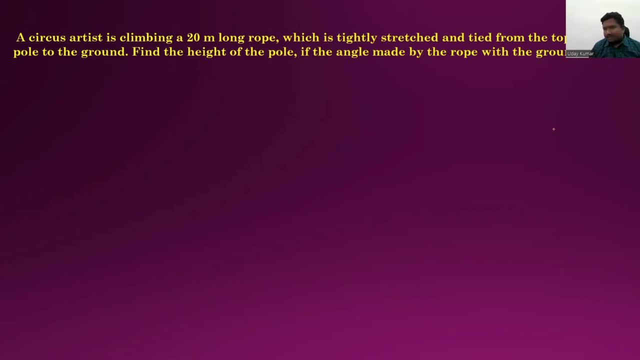 angle made by the rope with the ground level is 30 degrees. So after reading the question twice, I feel each and every point when we are writing the sentence relevant part of the picture. Again, the next sentence relevant part of the picture. 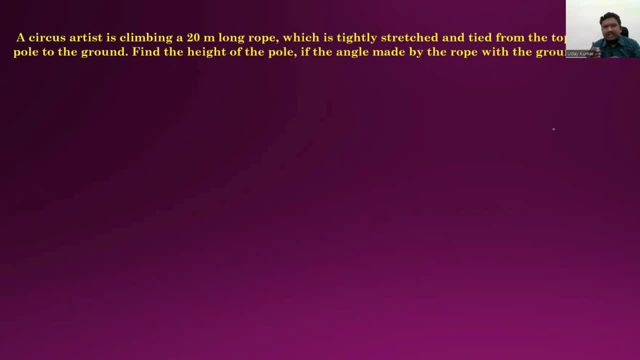 If we finish in such a way, we will not miss even a single detail in that and we can answer it very easily. We can understand even the question well, if you do in that way. So let us answer in such a way. So let us write the given information first. Given that height of a pole AB is equal, 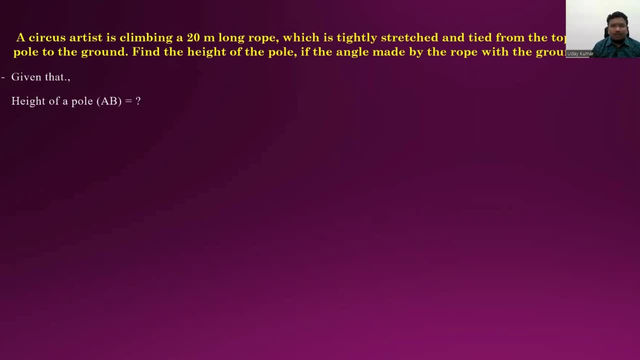 to question mark because they are asking us to find height of the pole that we do not know. Okay, So let us draw picture to that AB unknown. And next what we know: Length of a rope AC is equal to 20 meters, So where it is. 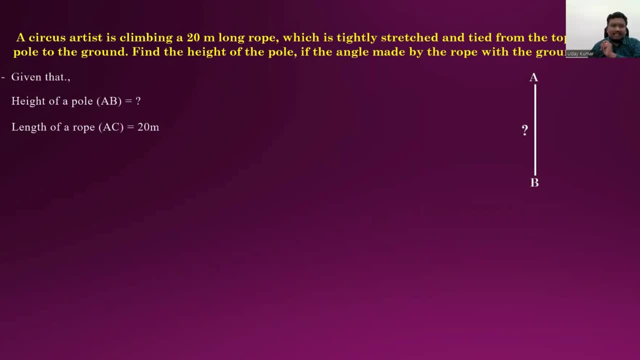 there, from the top of the pole to the ground. it is connected means tied, So AC is equal to 20 meters. Next, what we know Here, BC, whatever is there, AB is the pole, AC is the rope, Then BC. 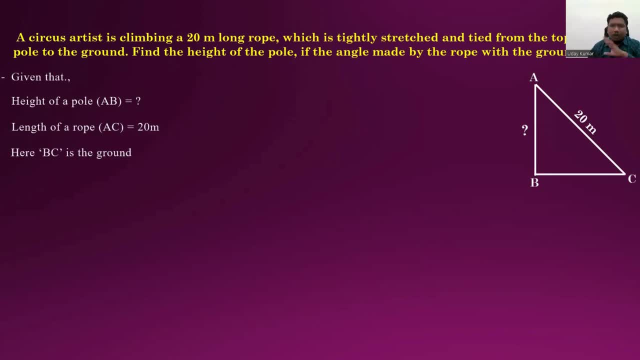 whatever is there. that is the ground. Here all are physical parts: Pole is there, rope is there, ground is there. So we have to use line segment only If it is any virtual part means which is not there. we are visualizing that We have to represent with the dotted lines. Okay, Next. 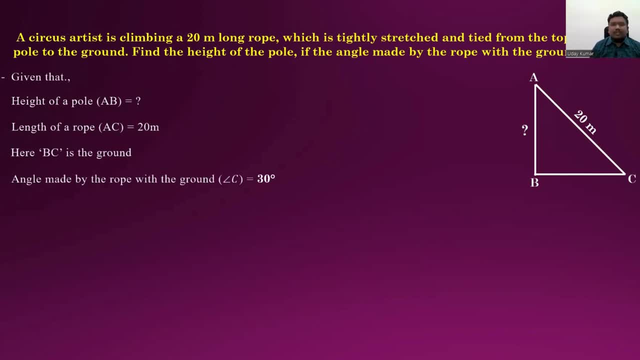 angle made by the rope with a ground angle, C is equal to 30 degrees. So here, where the angle is forming angle in between rope and the ground, there the angle is formed. Okay, So C is equal to 30 degrees. Next, here, what is happening? 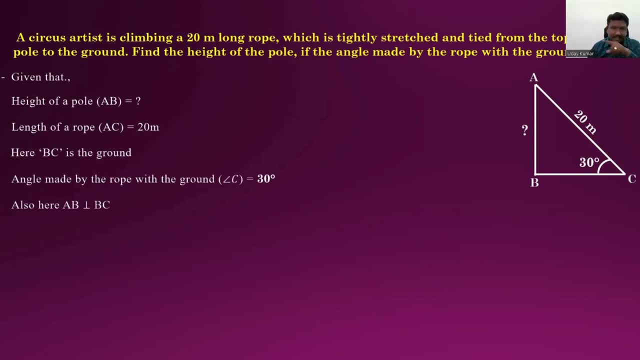 AB is perpendicular to BC means ABC is a right angle triangle. So we will mention even that. So till here, if you see, we wrote the whole information as a sentence and connecting picture. So picture part done, even given, information part done. Okay, Here we know about AC. We. 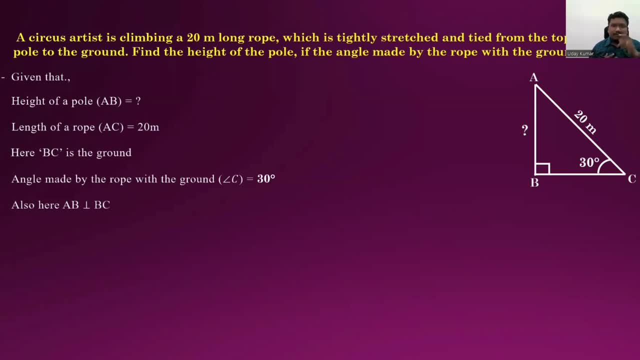 have to find AB. From which triangle ABC triangle? okay, From triangle ABC. Which triangle? Which trigonometric ratio is helpful for us? Just imagine to find the unknown AB using the known AC. So to that angle, 30 degrees. unknown AB is opposite side. known AC is the. 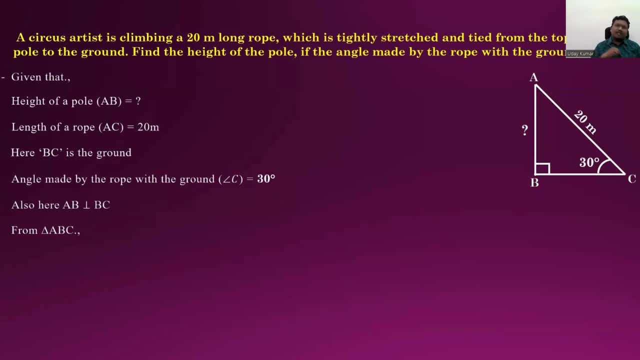 hypotenuse. So opposite side, hypotenuse related trigonometric ratio, correct sin. So let us apply sin theta there. Sin C is equal to AB by AC opposite side, by hypotenuse. Here what is the measure of C 30 degrees AB? we have to find AC 20 meters. Let us substitute: 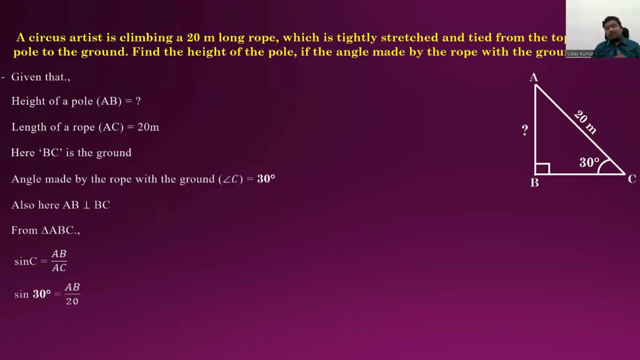 the values in it. Sin 30 is equal to AB by 20. and what about sin 30?? Sin 30 is equal to half. We substitute it Now from that. if you see, one half is equal to AB by 20,. 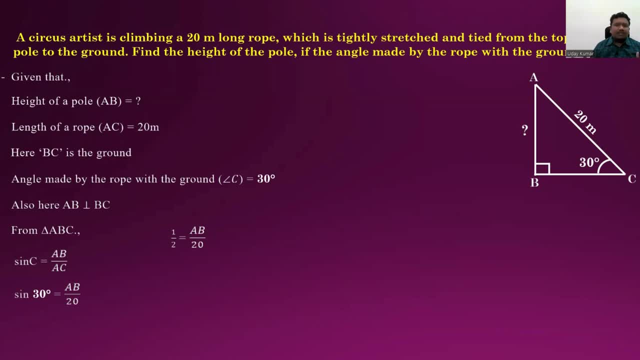 there 2 and 20. both are in denominator. we can cancel in two table, then finally we will get: AB is equal to, yes, 10.. 10 to 20, then AB is equal to 10 meters. So AB is the thing, what they are asking us. 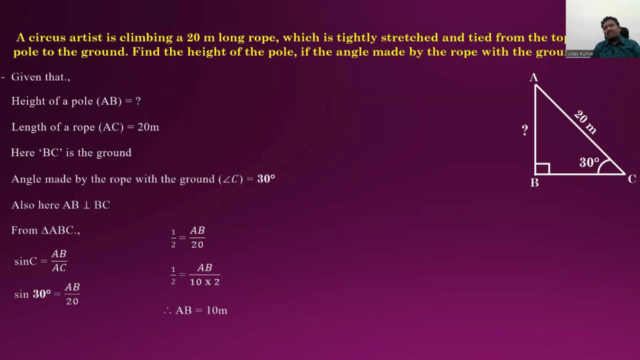 to find right. What is AB? Can I leave there itself? AB is equal to 10 meters. No, because according to my consideration, AB is the height of the pole. Maybe, according to your consideration, might be PQ, some other consideration, MN, like that. it may vary. So we didn't, we shouldn't. 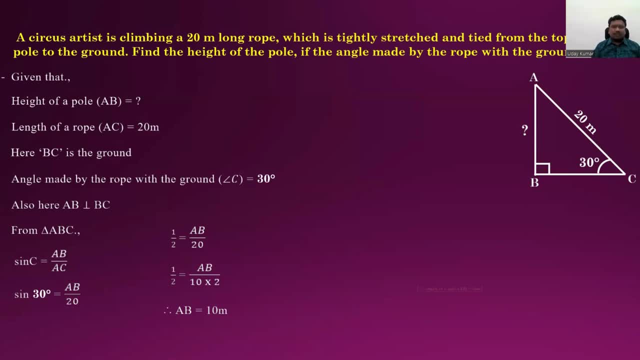 stop there itself. We have to give a conclusion. So what is the conclusion? Length of a pole AB is equal to 10 meters. Clear, Very simple. So reading the question twice, writing the information clearly accordingly, step by step: 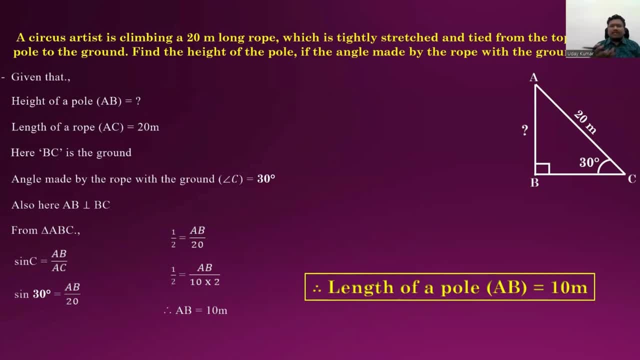 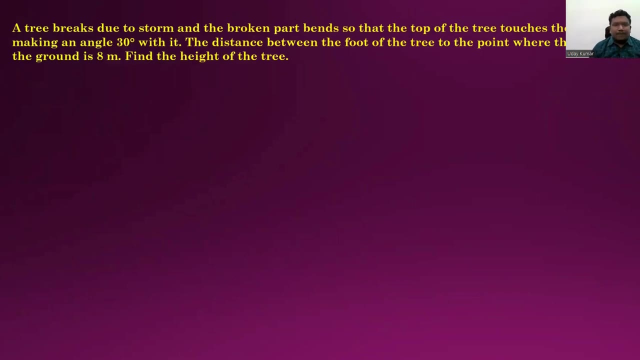 if you draw the picture, half of the task will complete. Then calculation part is just like that we can finish. So shall we enter into the next question Now? let us see the second question now. A tree due to storm, sorry, a tree breaks due to storm and the 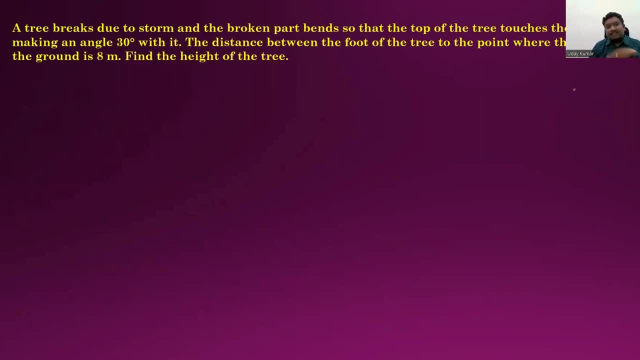 broken part bends, The top of the tree touches the ground, making an angle 30 degrees with it. The distance between foot of the tree to the point where the top touches the ground is 8 meters. So find the height of the tree. So height of the tree means you mean broken part, No. 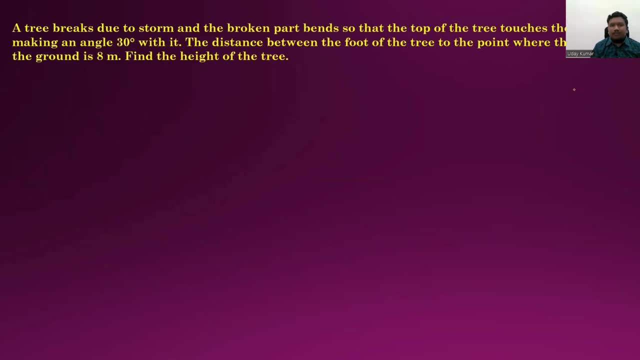 Before strong? what is the height That they are asking us? So let us see again what they are asking and what information they gave in the question. A tree breaks due to storm and the broken part bends, So that is where the top of the tree touches the ground, making an angle 30 degrees with it. The distance? 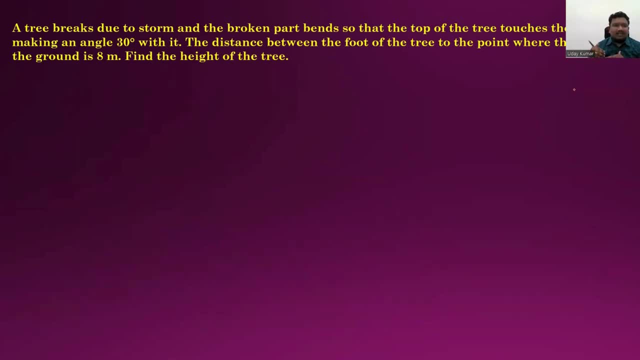 between foot of the tree to the point where the top touches the ground is 8 meters. Find the height of the tree. So we understood what they gave. Let us write the information given clearly, step by step. Also, let us draw the picture relevant to that. Okay, Right. 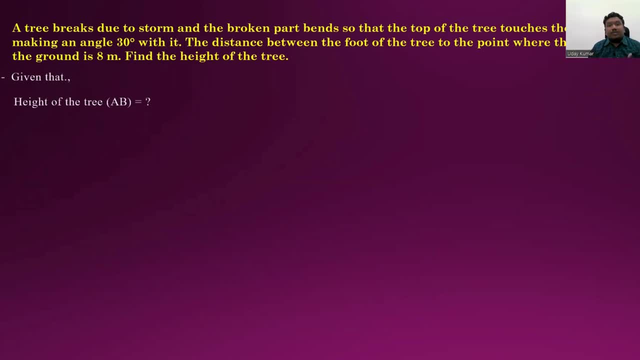 Given information, as usual. height of the tree A, B. We do not know. that is what they are asking us to find. So A, B is equal to 8 meters. So if you have a tree, the height of the tree is 8 meters. 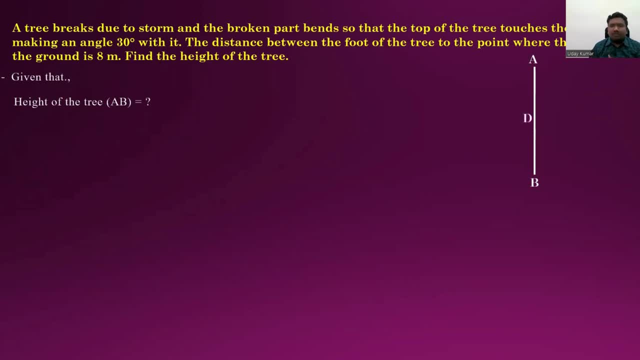 So the height of the tree is 8 meters. So we have to find the height of the tree So unknown, We do not know. What is D there? D is the point where, because of storm, tree was broken down. So now AB is original height, but after the storm, now it is only DB. That 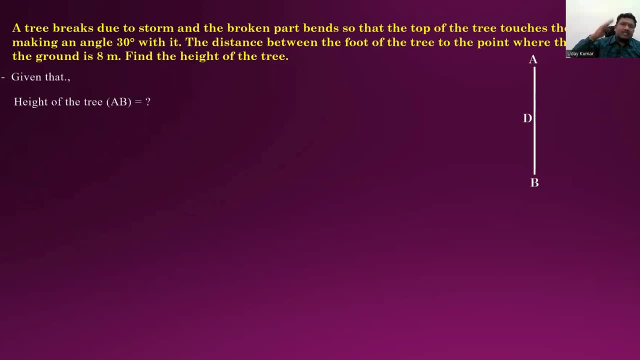 AD part whatever is there that was fallen down. Now that is touching the ground. Okay, So that information we will write. Length of the broken part, DC. If you mention that as C, then this is the situation: That AD whatever is there that will become PC now. 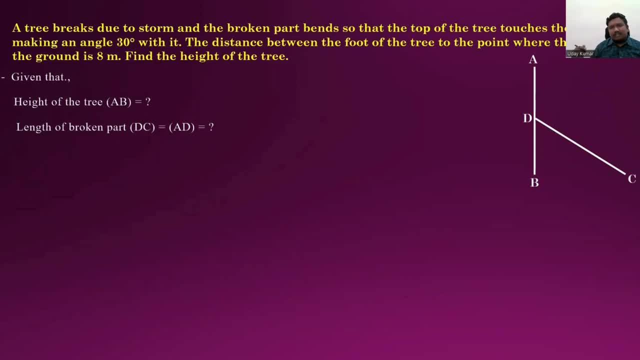 That will become DC. So length of AD, length of DC, both are the same. We can't use CA again there because the same letter we can't repeat in the question. So that's the reason I took it as C. Now that we have to find DC, we have to find because DC is nothing but. 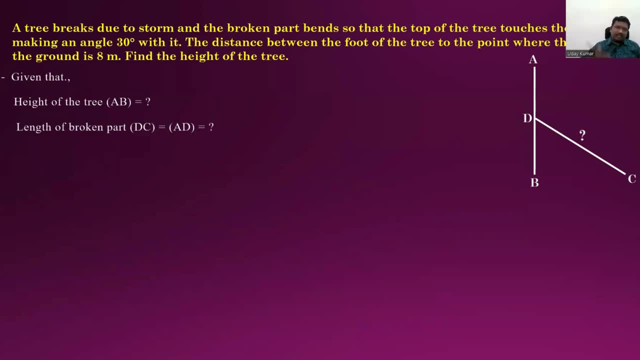 AD. If I find AD and BD automatically, I can find the height of the tree actually before the storm. Okay Now distance between foot of the tree and top of broken part. So top of the broken part is C and foot of the tree is B. Between those two, whatever is there BC, 8 meters. 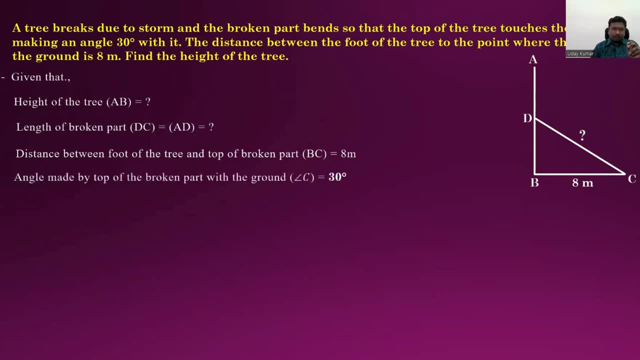 Next, what we know here: angle made by the broken part with the ground. Now broken part means DC. Actually it is AD, Now it is DC. That top of the broken part means C with the ground. How much angle it is making? They told very clear it is 30 degrees. So 30 degrees. 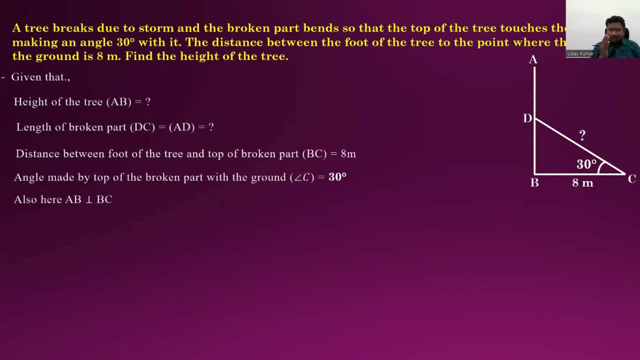 let's mention the picture even Now here. if you see that broken part after the left out part, whatever is there, that means DB and the ground BC. both will make an angle 90 degrees. That's what mentioned here. Let us mention even in the picture. Okay, Next, So we have. 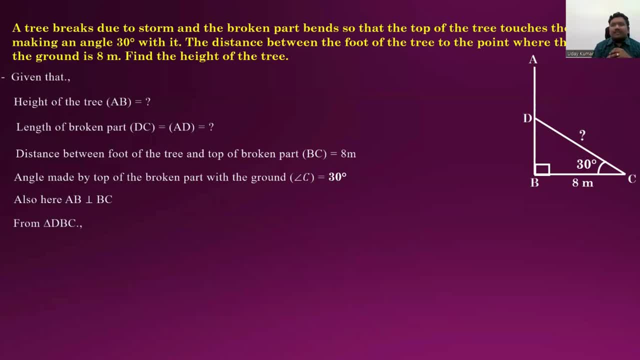 DBC. So we got DBC, which is a right angle triangle, In that right angle triangle. I don't know DB, I don't know DC. Both I have to find Stepwise. let us find. Okay. So first cos C. Cos C means adjacent side, What I know, adjacent side, what I have to find DC is a. 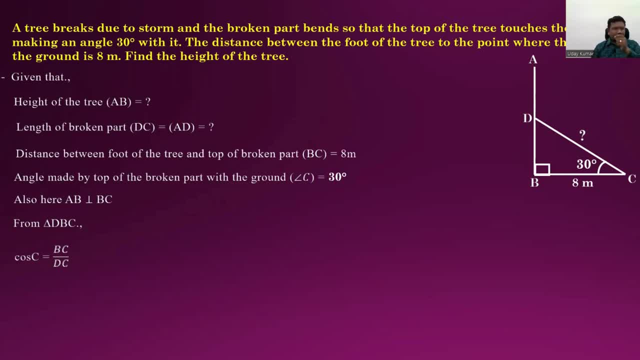 hypotenuse Relation between those two is cos C. Here, what is the measure of C 30. Cos 30.. Cos 30, how much 30. Okay, It's root 3 by 2.. Sin 16: nothing but cos 30. So we'll substitute that Whatever. 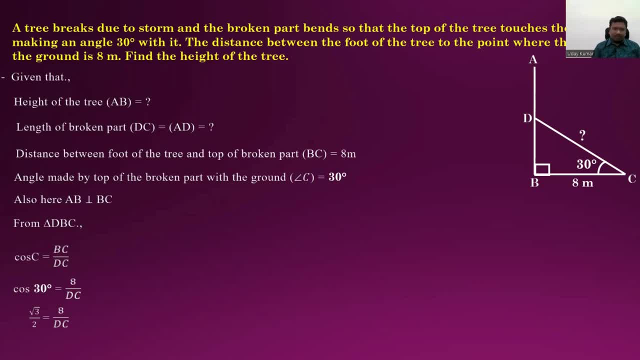 we know we'll substitute and we'll simplify that From there. what we get it is 16 over root 3.. DC means 16 over root 3 after doing cross multiplication And I got DC, which is the broken part. That is not sufficient right To find height of the tree we need. 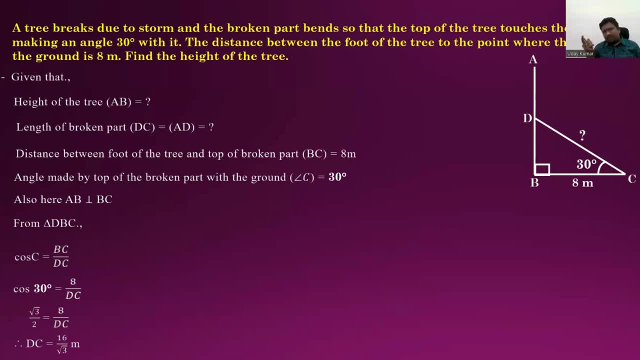 to find even DB also. Now that DB is what? according to the angle, opposite side. Now I know I have to find opposite side, I know adjacent side. I now hypotenuse, So I can go with either sin or tan, Anything we can. Okay, I will go with tan, opposite, adjacent. 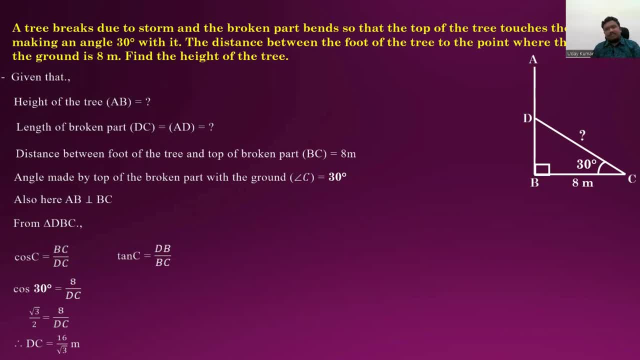 Adjacent means 8 cm, 8 meters BC. Opposite means BD, which I have to find. So let us substitute Tan C, tan 30.. Tan 30.. How much? Yes, it is 1 over root 3.. Correct, 1 over root 3.. So. 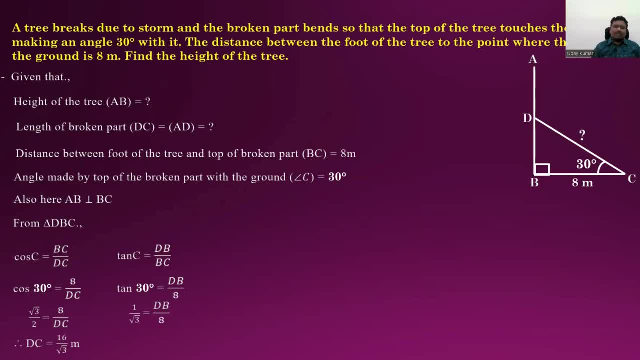 root 3 is equal to db by 8.. Even here let us do cross multiplication so that we get db is equal to 8 by root 3.. dc 16 by root 3. broken part db means the left out part is 8 by root 3. Those 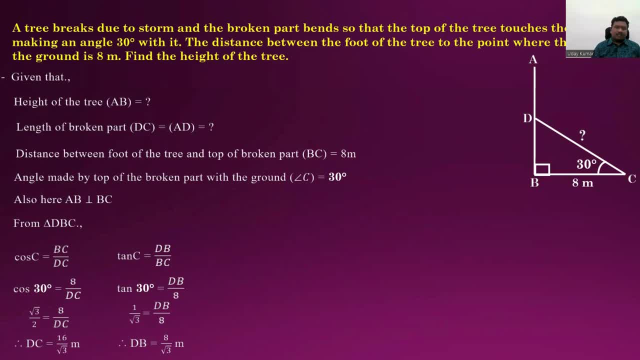 both. if we add that is nothing but height of the tree, right? Let us do the same. Height of the tree. ab is equal to db plus dc. Okay, So now dc, how much db? how much? 8 root 3? 16 root 3. I substituted. 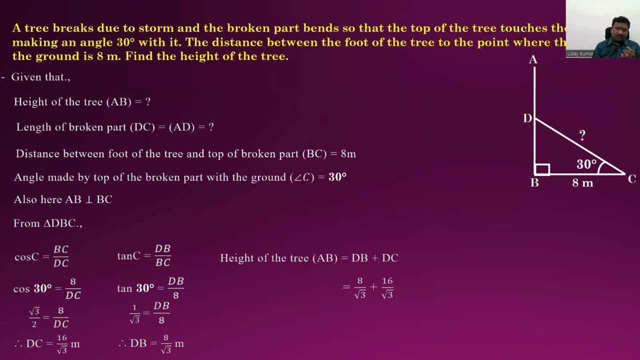 in that. Now let us simplify. Those are like fractions 8 by root 3 plus 16 by root 3, 24 by root right, So 24 by root 3.. Shall we leave here itself, Especially in the denominator root is. 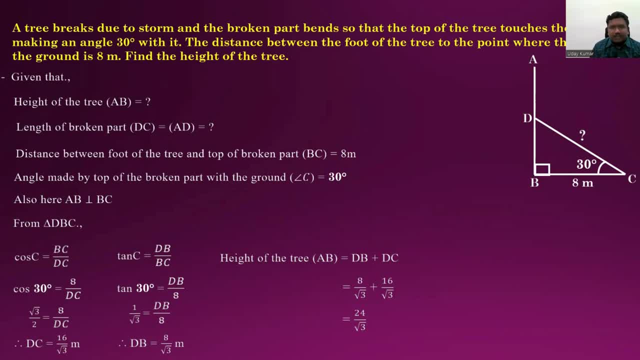 there. That shouldn't be the final answer. We have to rationalize, or else I can write that 24 as 8 into root 3, into root 3.. So that root 3 gets cancelled And finally I will get 8 root 3.. Because 24 is nothing but 3 into 24.. 3 is nothing but root 3 into root 3.. 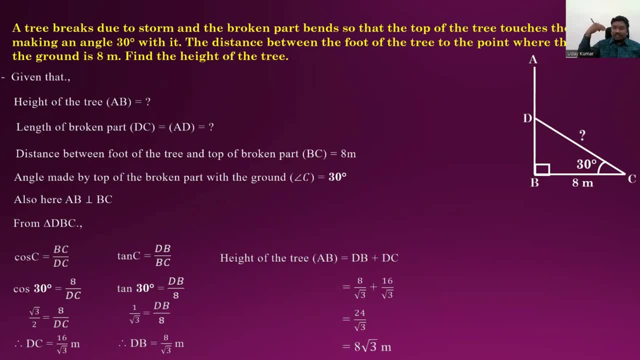 If I write like the denominator root 3, numerator root 3 gets cancelled. Still one more: root 3 is in the numerator along with 8.. That will become the final answer. that is actually height of the tree. So, as usual, we can't leave here itself. We have to rationalize. 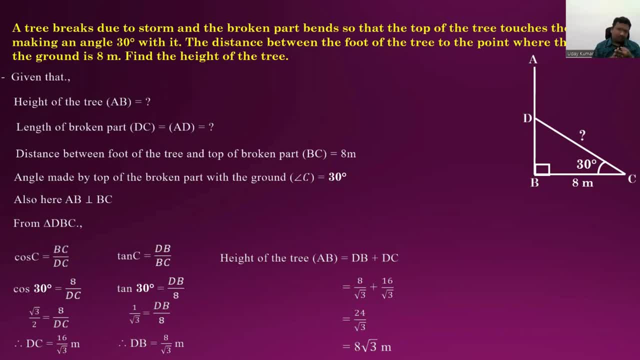 the conclusion. You know that, given information, picture process, conclusion Conclusion also very, very important while we are answering the question to get full marks. So let us write the conclusion. Height of the tree AB is equal to 8 root 3.. So simple, Very important. 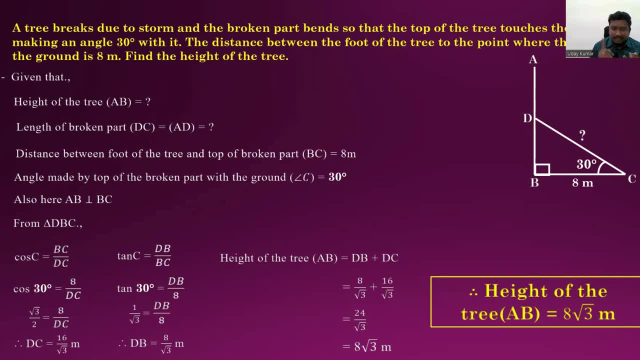 question. So we discussed the first one. Hope you understood very clearly. Second one as well. Till here I think you understood the concept very well, Even how we have to draw the picture, how to write the sentences. I think you are very much clear with this session. 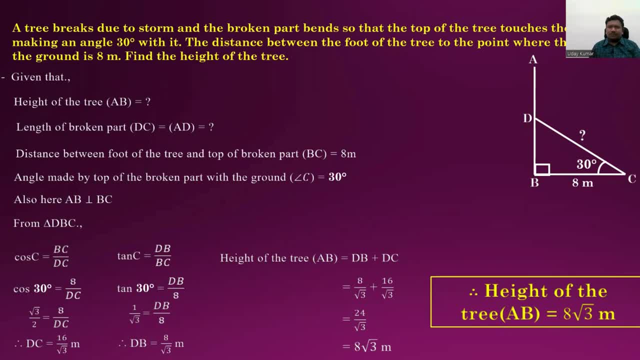 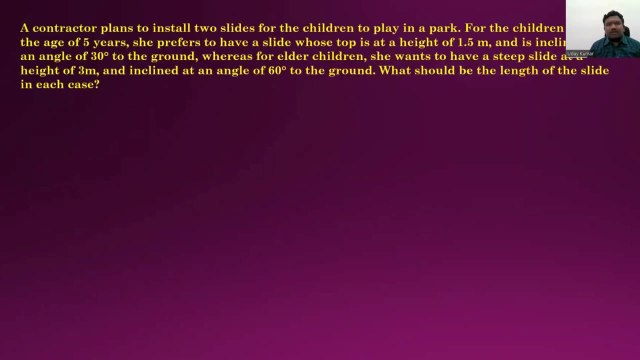 Right, Really, if you like to hear this video, what you have to do, You know that Right, Please do that. Okay, Now let us do. third question of the third session. Okay, A contractor plans to install two slides for the children to play in a park For the children below. 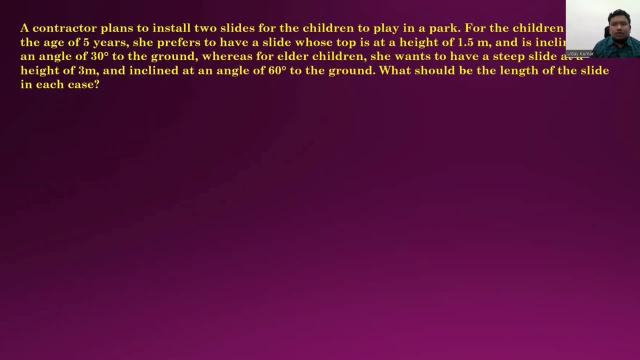 the age of 5 years. she plays in a park For the children below the age of 5 years. she prefers to have a slide whose top is at the height of 1.5 meters, means 3 by 2 meters- and is inclined at an angle of 30 degrees to the ground. whatever is there, that slide which is 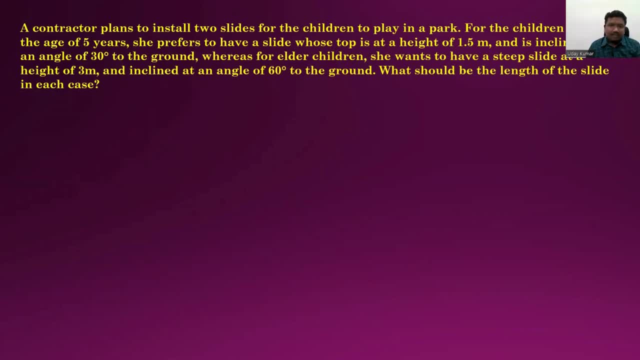 preferred for the children age of 5 years. below 5 years, that is making an angle 30 degrees with the ground, whereas for elder children- so with elder above 5 years- she wants to have a steep slide at a height of 3 meters. so altitude is difference. for small children, toddlers it is. 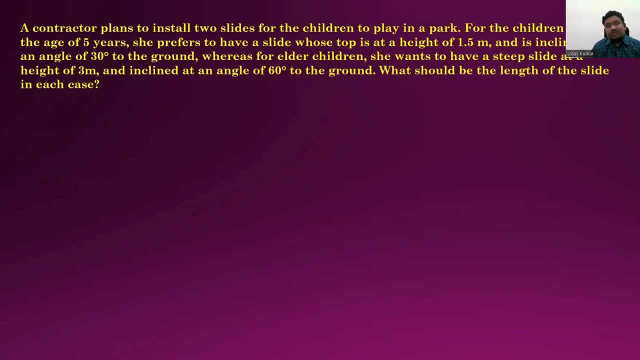 only 1.5 meters, whereas for the elders that is 3 meters tall and inclined at an angle of 60 degrees. she can't maintain the same angle right because it is too tall, double of that. automatically, angle of elevation also will change. so that is 60 degrees now. what should be the length of the 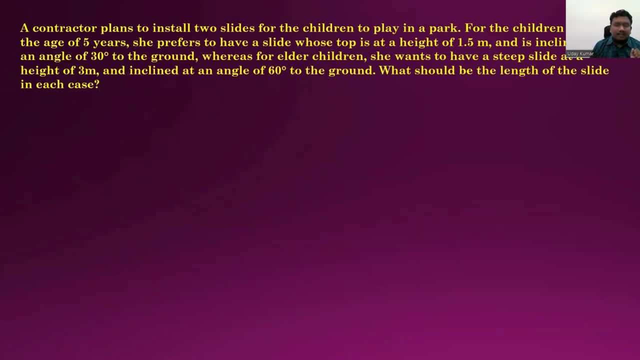 slide in each case, both the slides. height of length we have to find, not height, height means altitude, that is already given length. So first let us write the information, followed by the picture along with it. so let: abc is a slide inclined at 30 degrees, with ac means abc triangular shape, in that ac is the slide, ab is the altitude. 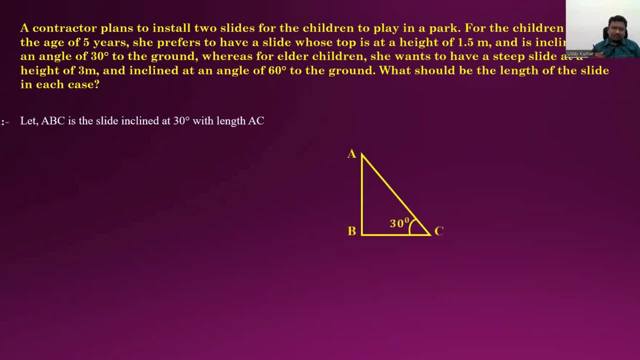 of the slide maintained with the ground. that picture, ab is the altitude, ac is the slide. slide is making an angle 30 degrees with the ground. Now about another slide, the slide which is for elders, for elders, pqr am constipate. pqr is a slide. 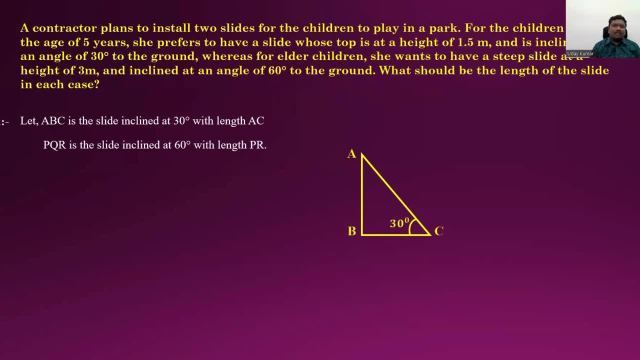 inclined at 60 degrees with length. pr means pr is a slight length, pq is the altitude or height maintained by the slide from the ground. that is the picture. so here, in this case, what we have to find, we have to find ac and pr. okay, right. 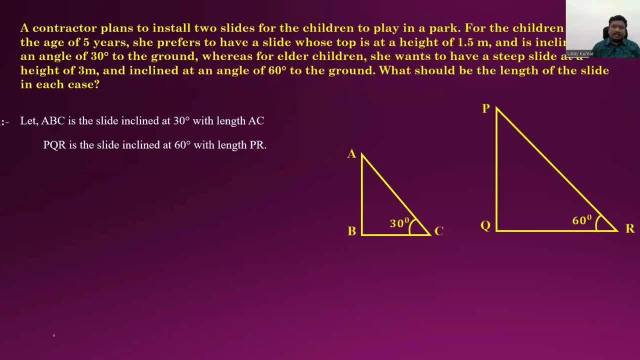 Thank you very much. We know already AB as well as PQ In this triangle. ABC, what we know? We know that sin 30 degrees is equal to AB by AC. Do we know AB? Yes, we know AB, half they already gave. 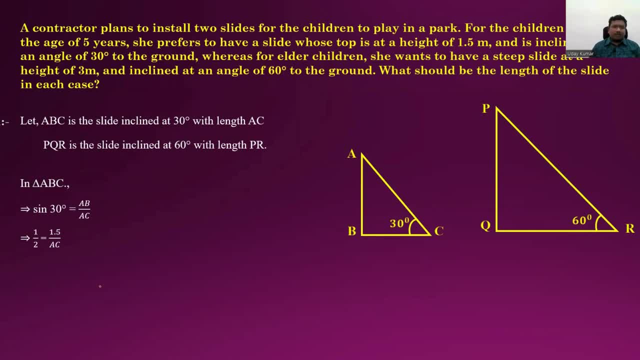 that, which is 1.5 meters. 1.5 meters they gave, and we know that sin 30 is equal to half. We substituted from that What is the measure of AC? If you do cross multiplication, AC is equal to 3, which means length of the slide allotted for the children below 5 years. Now, 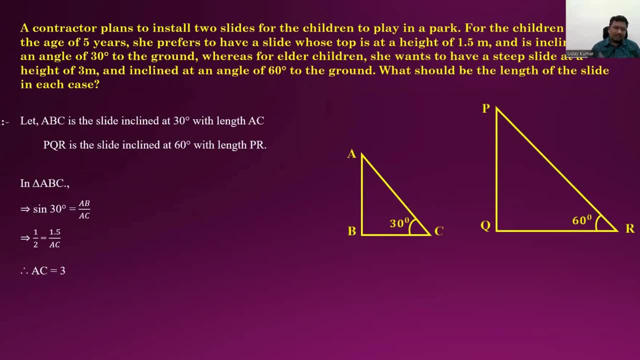 let us find PR. PR is the slide allotted for the elders, elder children above 5 years. So there also allotted the same thing, sin. So. but in triangle PQR, sin 60 is equal to PQ, opposite side, PR, hypotenuse. So sin 60, how much Root 3 by 2.. So root 3 by 2 is equal. 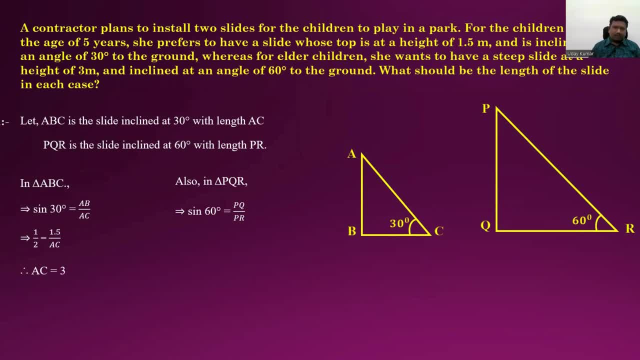 is equal to P Q. how much 3 meters? So we will substitute those values From that. if we do cross multiplication, what we get P? R is equal to, yes, 2 root 3.. How can we get 2 root 3?? They are actually. 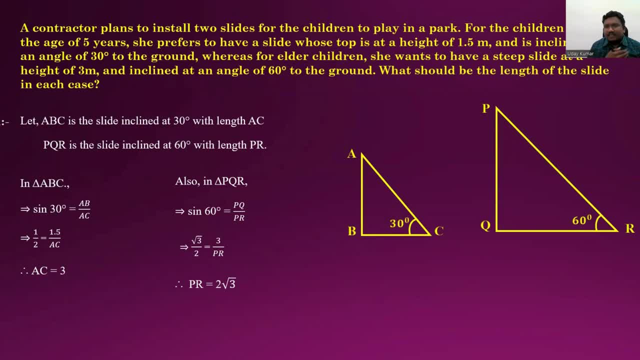 6 over root 3.. 6 over root 3. if we simplify, just like earlier question, here I just wrote in a direct way: 6 over root 3.. 6, nothing but root 3 into root 3 into 2.. So root 3, root 3 gets cancelled. 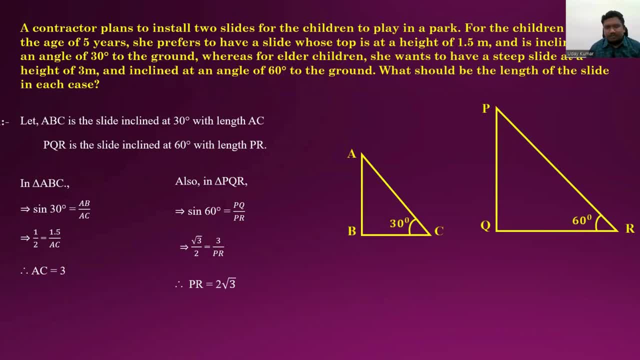 and we will get 2 root 3 finally. So can we leave here itself. A C is equal to 3 meters, P R is equal to 2 root 3 meters. is that ok? No, you know that you have to write the conclusion, So let us write. 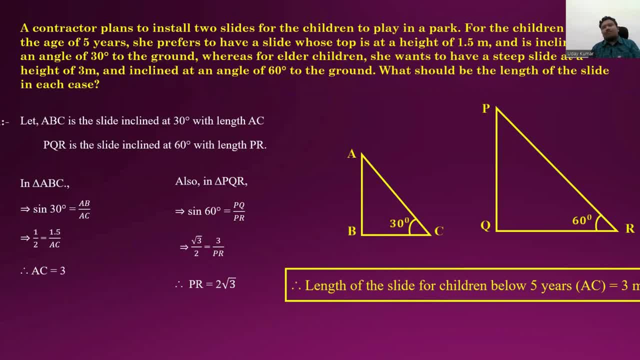 the conclusion. So length of the slide for the children below 5 years: A, C, 3 meters. Similarly length of the slide for the children below 5 years. So length of the slide for the children. length of the slide for elder children: P R is equal to 2 root, 3 meters. ok, So similarly even. 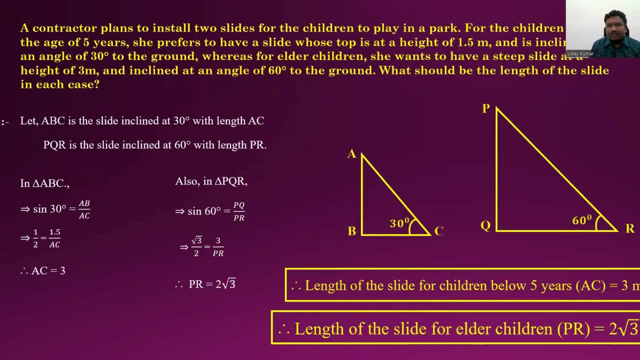 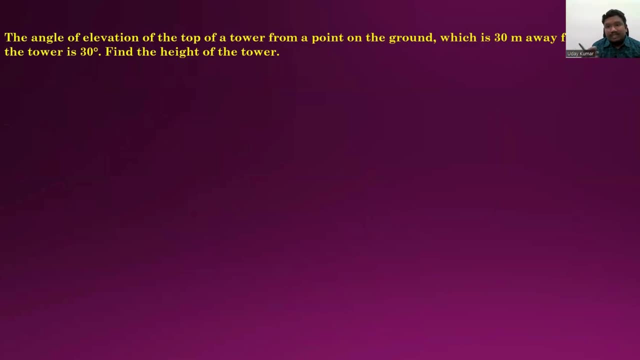 fourth question. fifth question also we will discuss in this session Till fifth question we are going to discuss in this video. ok, Shall we move to the fourth one: The angle of elevation of top of the tower from a point on the ground which is 30 meters away from the foot of the tower. 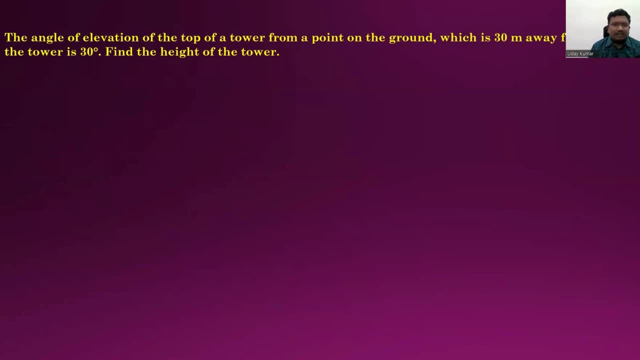 is 30 degrees, Find the height of the tower. So here it is very much clear: there is a tower, there is a point observer. From that point they are observing the top of the tower with 30 degrees and that distance, which is 30 meters away from that that point observer, whoever is there, 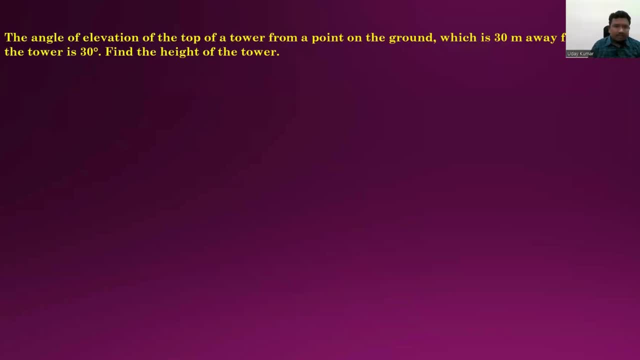 maintaining 30 meters distance from the foot of the tower. ok, Now here we have to find height of the tower, where is simple right angle triangle picture will come. So, given that, as usual, height of the tower, they are asking height of the tower, So I generally I prefer 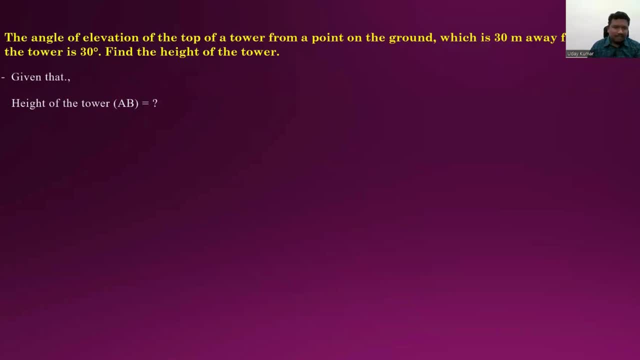 to take AB only as a height of the tower, So that we have to find here. So AB is equal to question mark. we don't know. Next, distance between foot of the tower and point observer BC. So there is a point, observer C, from where they are observing top of the tower. ok, So 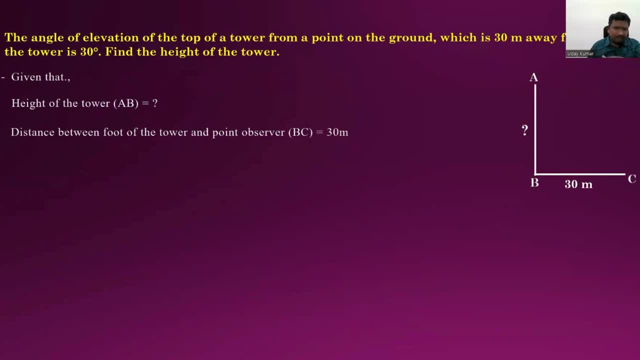 that is the distance from C to B, distance between foot of the tower and point observer: 30 meters. Next, what Angle of elevation? See, till now there is no angle of elevation. Question number one. question number two, question number three, if you observe. 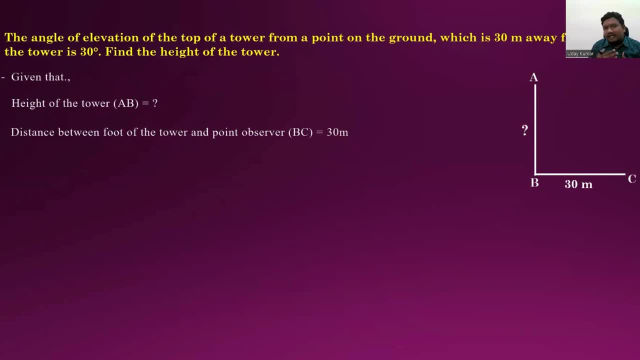 there is no discussion of angle of elevation, There is only angle made. but here, for the first time, angle of elevation is there because person is observing which is actually not there, Just we are visualizing them. So when we are visualizing we cannot give the same marking. we will use the 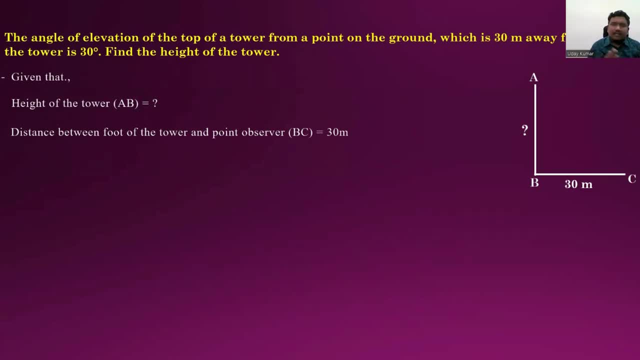 dotted lines. You know that. So with the dotted lines, especially as it is angle of elevation, we have to mention even the arrow mark upwards. So angle of elevation from the point observer c is equal to 30 degrees. That is the picture. So we got complete right angle triangle. Oh, we did. 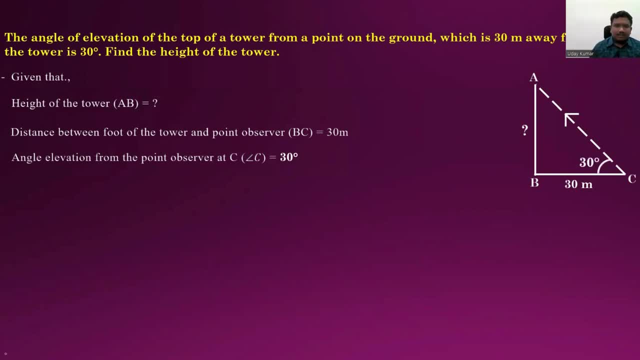 not mention the 90 degrees. So let us mention even that 30 degrees angle of elevation. Also here, a b Perpendicular to b c. Let us mark even that Now we got complete right angle triangle picture in which I know b c. I have to find a b, A b, I have to find which is opposite side to the theta. 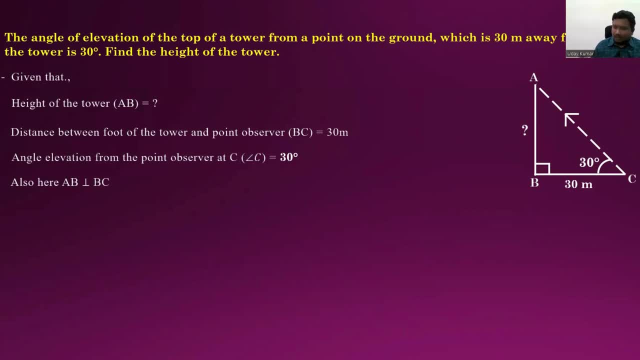 b c, I know, which is adjacent side to the theta, Opposite adjacent relation, tan. So let us apply: So from triangle a, b c, tan c is equal to a b opposite side, by b c adjacent side, tan c, tan 30. So let us substitute the values, what we know. 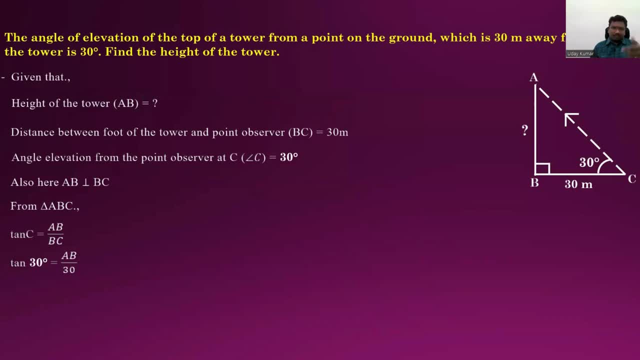 tan 30 is equal to a b by b c. We know already b c That we mentioned there. Next, tan 31 by root 3 is equal to a b by 30. Now let us do cross multiplication. It will become 30 by. 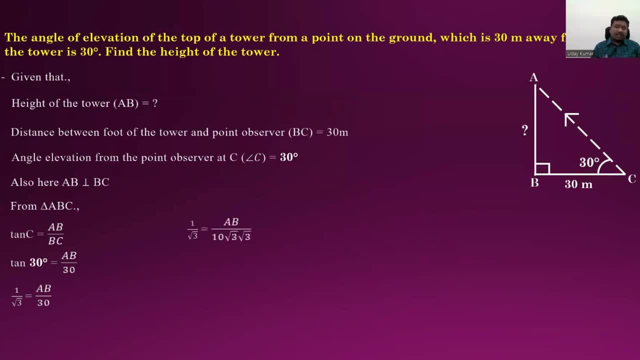 root 3.. a- b is equal to 30 by root 3.. But I do not want to represent like that Easy process 30 if you write it as a 10 into root, 3 into root 3.. Because root 3 into root 3 means 3.. So there itself. if we cancel that, then here LHS denominator. 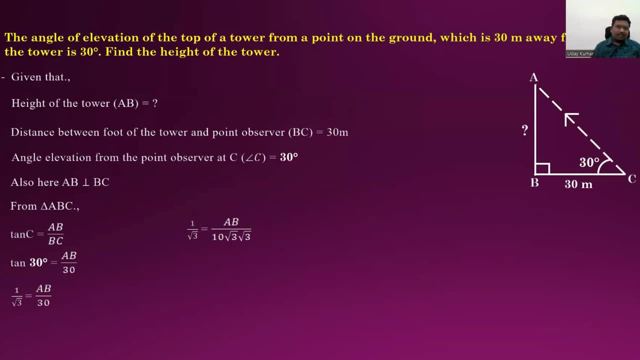 root 3. RHS denominator root 3 gets cancelled. Finally we will get: a b is equal to 10 root 3, if I do cross multiplication. But what is a b? Height of the tower? Let us mention the conclusion part. Yes, Height of the tower, a? b is equal to 10 root 3 meters. It is not 10 meters, It is 10 root. 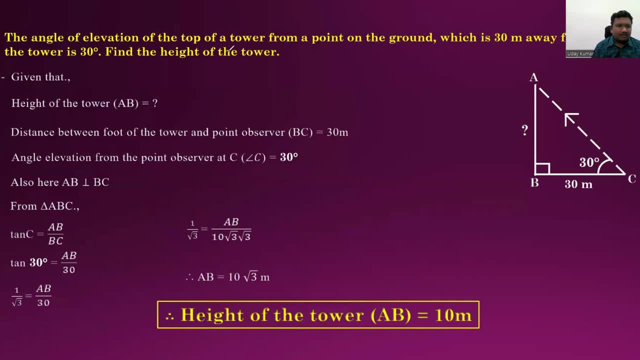 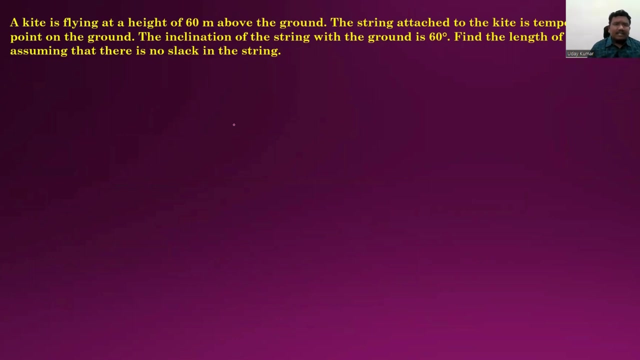 3 meters. This is 10 root 3 meters: 10 root 3 meters. Okay, Right Now. next fifth question: A kite is flying. height is 60 meters above the ground. The string attached to the kite is temporarily tied to the. 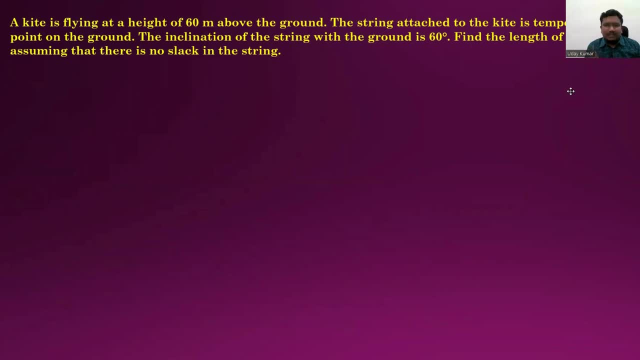 point on the ground. The inclination of the string with the ground is 60 degrees. Find the length of the string, assuming that there is no slab in the string. So what does it mean? there is no slab Means no knots, nothing. Completely straight. The string is completely straight. So they are asking: 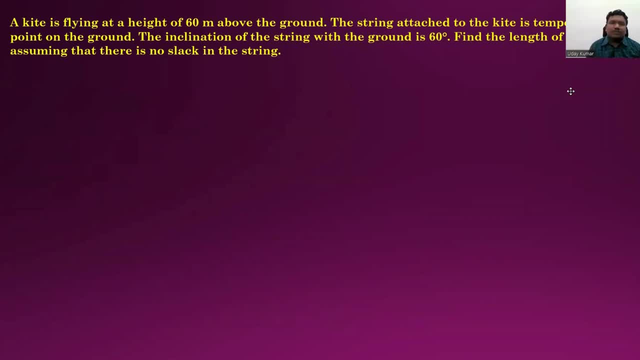 length of the string. Length of the string means automatically hypotenuse. Hypotenuse We have to find, and they gave height of the kite. actually it is not height of the kite. altitude, how much altitude that kite is maintaining is simply generally what we call. that is height: 60 meters. 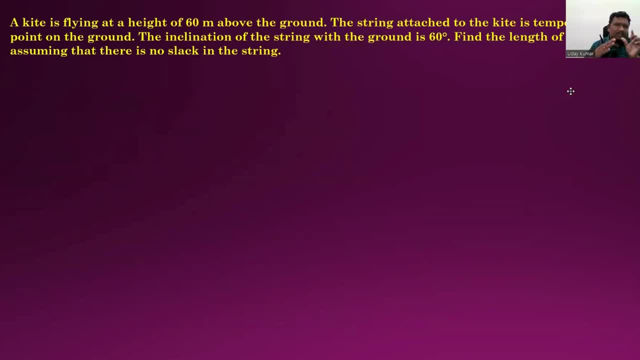 they gave, and length of the string they are asking. so opposite hypotenuse sign we have to apply. okay, so firstly let us write the information, what they give. given that altitude of the kite, how much, uh, altitude that kite is making? 60 meters it is making. so we'll draw the picture. 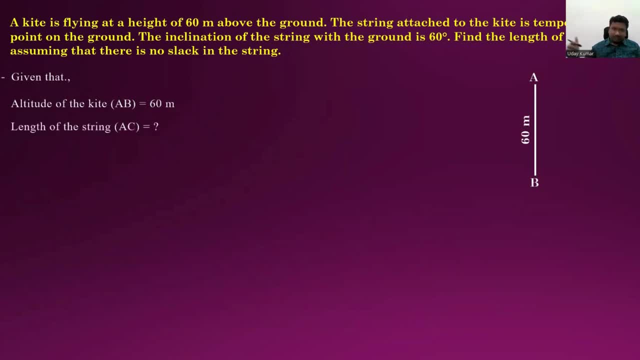 followed by length of the string. that is also there. so should i use the dotted lines or line segment, line segment, right, okay, next, bc is just a ground. ab is altitude maintained by the kite, ac is the string. bc is just a ground, just a connected, a joint, now angle made by the 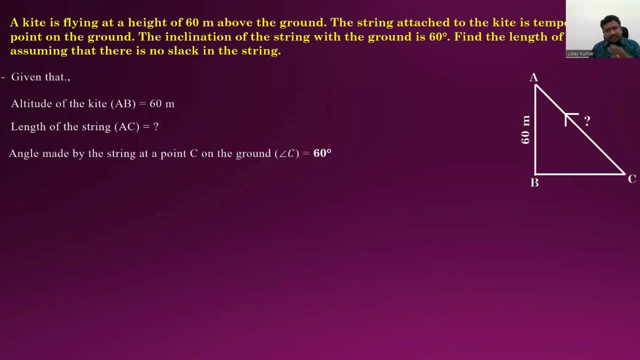 string at a point c on the ground, how much angle that string is making. they gave very clearly in a question: it is 60 degrees. 60 degrees next also here: ab bc. they are perpendicular to each other always. they need not mention we have to write ab perpendicular to pc. okay, 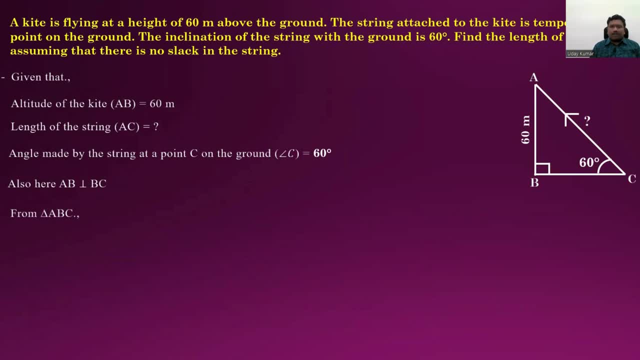 now abc is a triangle, as i told you. we know opposite side. we have to find hypotenuse first, so opposite hypotenuse related trigonometric ratio. sine theta. substitute that sine c is equal to ab by ac. sine c means sine 60 is equal to 60 by ac. 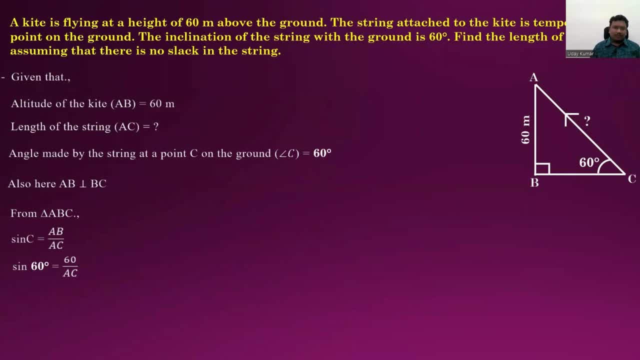 sine 60. how much root 3 by 2? so root 3 by 2 is equal to 60 by ac. then accelerate 60 as 20 into root 3, into root 3, so that it will get cancelled. root 3: root 3 gets cancelled. 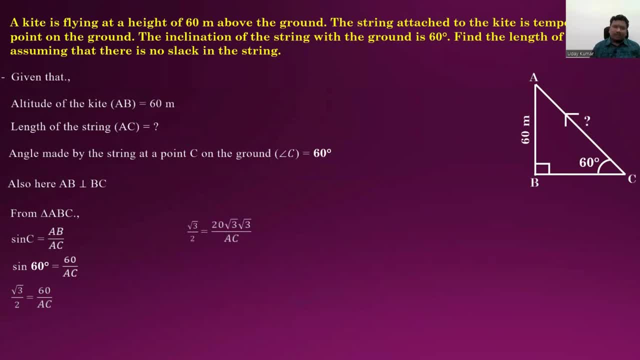 then i will do cross multiplication. then i will get ac is equal to 40 root 3, so automatically ac. what they are asking is length of the string. so length of the string is equal to 40 root 3 meters. okay, hope you understood these all questions very clearly. 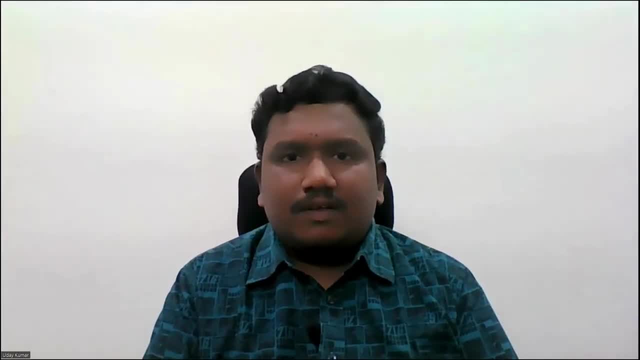 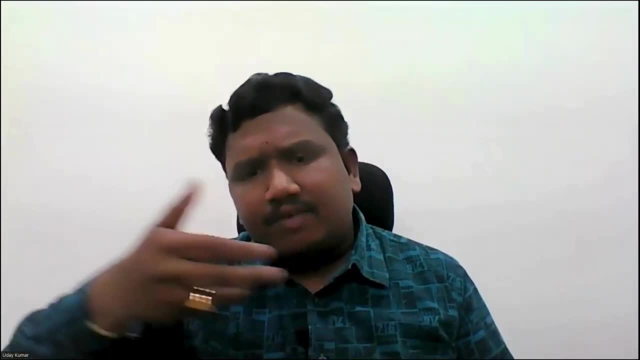 can i consider that? yeah, so if i have a string of 40 root 3 meters, then i will get. ac is equal to 40 root 3 meters. so if not, if you want suppose one more view, better have a look of the whole session then.